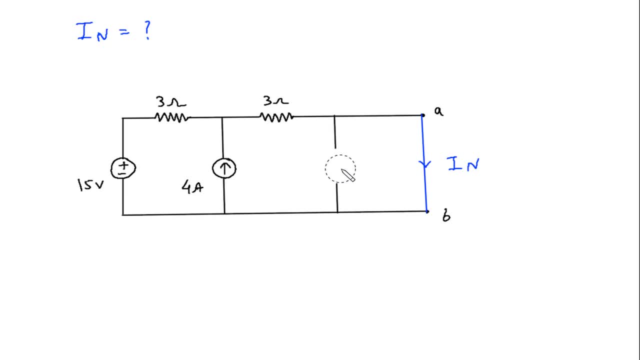 This 6 Ohm resistance will become 0.. Now let's assume this is node V1.. Let's assume the direction of current. Let's say this is current I1.. And this is current In Apply KCL at node V1.. 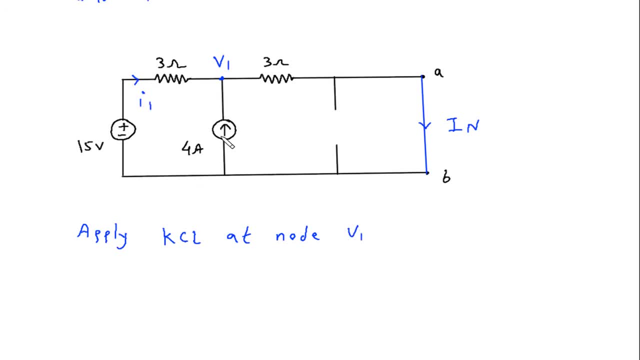 So at this node we will apply KCL Summation of all the entering current. Entering current is I1 plus 4.. Is equal to leaving current is In. This is our reference node, So I1 is equal to 15 minus V1.. 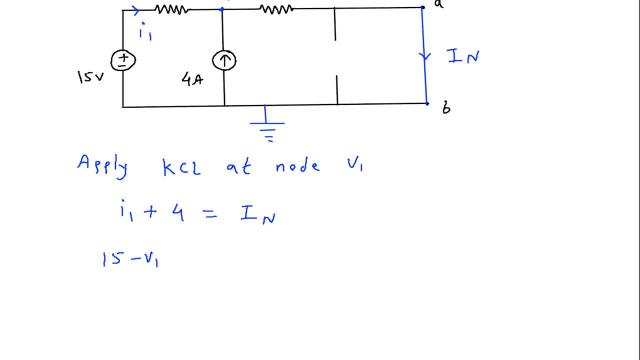 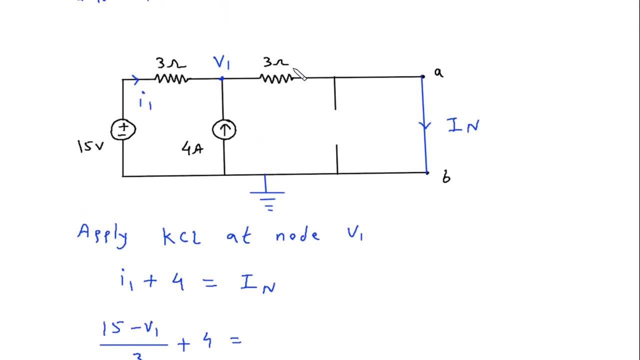 15 minus V1 by 3.. Plus 4 is equal to In. Now In is equal to V1 minus 0 by 3. V1 minus 0 by 3.. So this will be 15 by 3. Minus V1 by 3.. 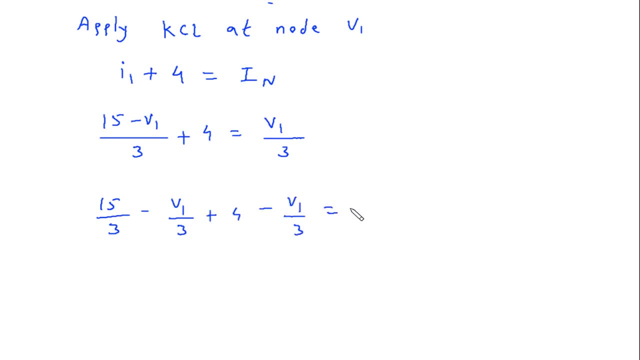 Plus 4 minus V1 by 3. Is equal to 0. So this will be 5 minus V1 by 3.. V1 by 3. Plus 4 minus V1 by 3. Is equal to 0.. 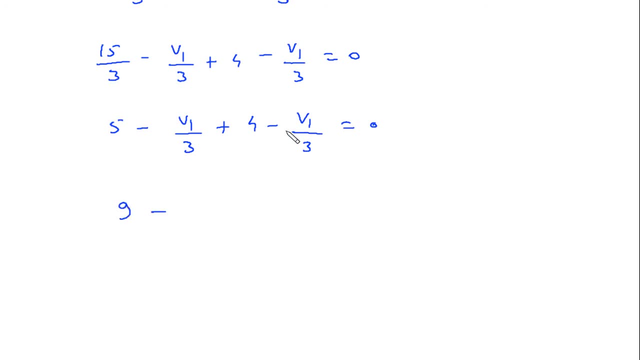 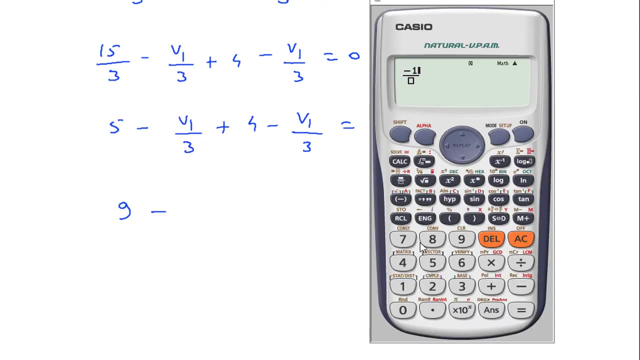 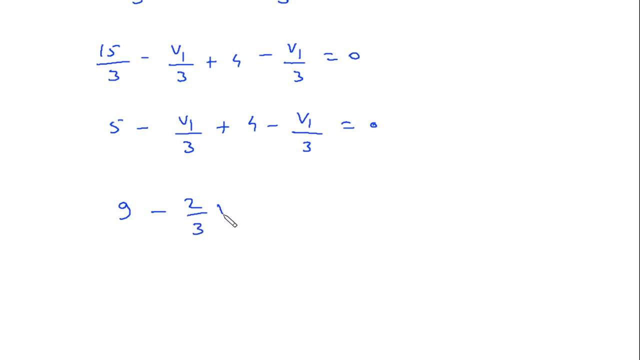 And this will be 5 plus 4, 9. Minus, minus, minus, Minus 1 by 3.. Minus 1 by 3. Minus 2 by 3. V1 is equal to 0.. 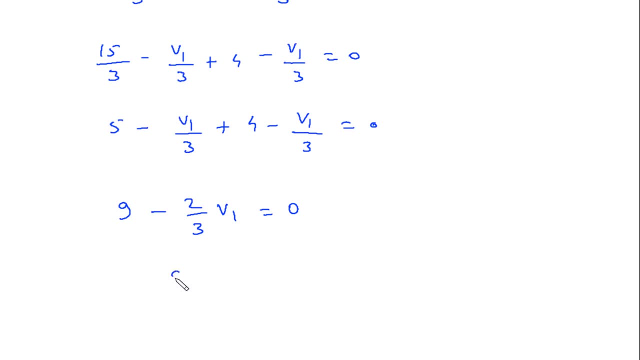 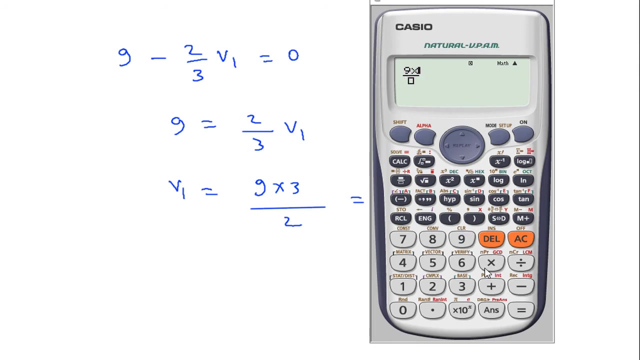 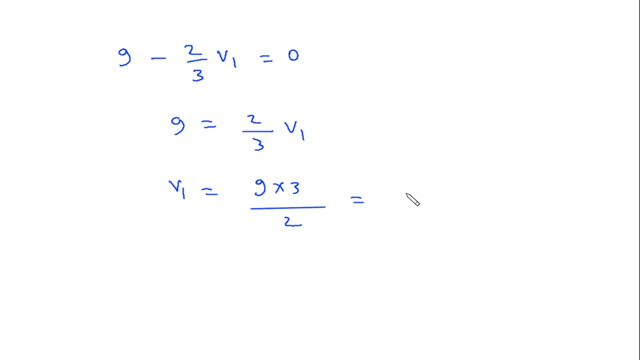 So this will be minus. or 9 is equal to 2 by 3. V1.. So V1 is equal to 9 into 3 by 2.. 9 into 3 by 2.. 13.5.. 13.5 volt.